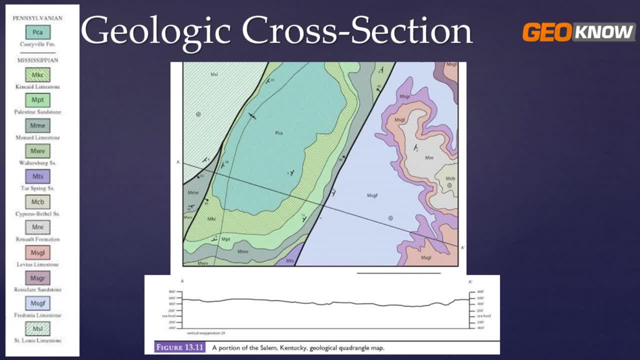 Hello everybody. this is Matt here. Thank you so much for watching GeoKnow. Today I'm going to show you how to construct a geologic cross-section. So here in front of you, you see a map, and this is just an aerial view. So if you're flying over the area in an airplane, you'd be able to look. 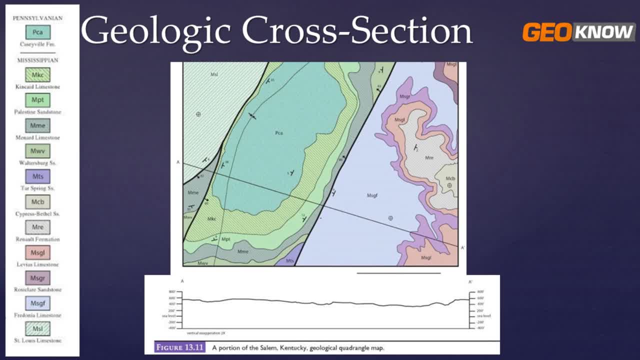 down and see this, Except, of course, we've delineated, or someone has gone out and mapped, the different geologic rock units, So we've got those here. We've also got dip directions and a few other bits of information that I think will be useful to you. 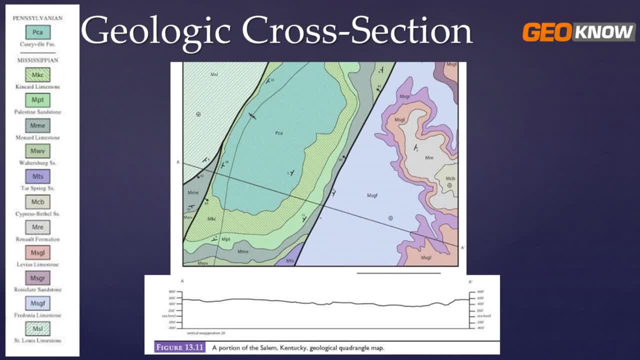 And I'm actually pretty excited to teach this, because when I was first starting- I feel like I was just it was just kind of expected that it would make sense and anyone would be able to figure it out. But I don't think that's the case. It's not that straightforward, It's not that common. 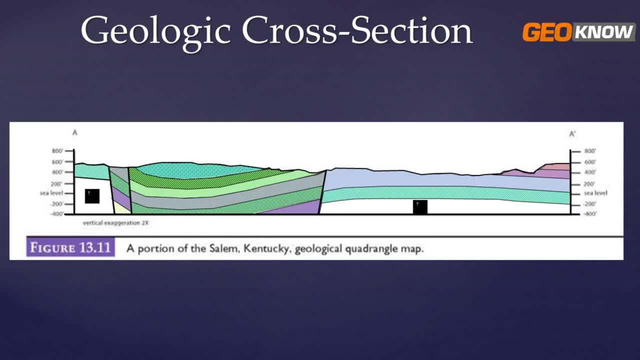 sense, I don't think The first thing is just what is a geologic cross-section, And I think the best way I could do to describe that is: it's kind of like a road cut And if you look at a piece of cake you'll be able to get a good idea of what a geologic cross-section is. 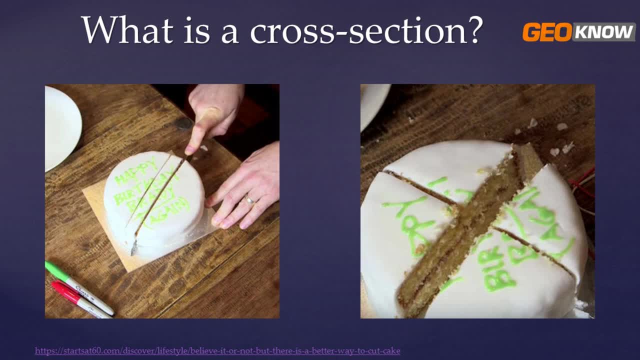 So picture that first picture on the left as the cross-section line, one of those, the cross-section line that you're asked to draw, And then the picture on the right. you can actually see down a vertical surface, you know, basically depicting what's going on. 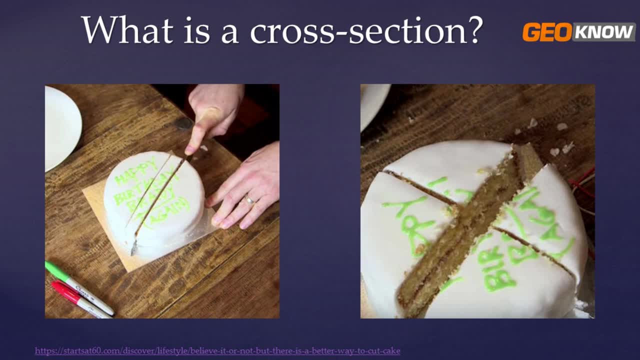 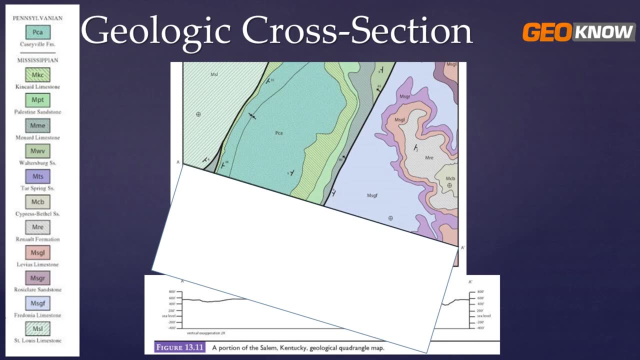 underneath the ground. So that's what a cross-section is. So if you cut a piece of cake and you look at the slice, that's a cross-section In the geologic world of things. think about this line A to A prime as where you're going to cut the cake. So we're going to take a big knife and 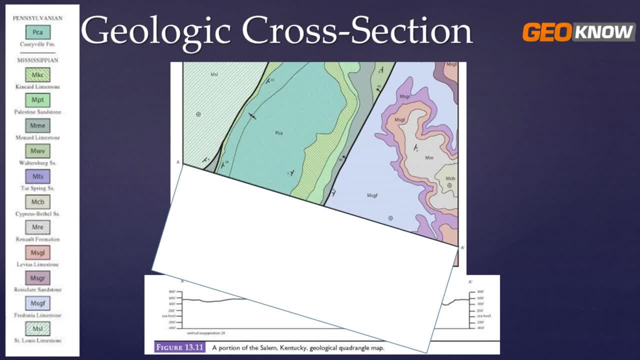 cut along this line and then take it away and see that vertical surface, see what's underneath the ground there. And the best way that I've found to do this is just take a piece of paper and place it along that line A to A prime. And every time you go along that line, either left to right or right to left- 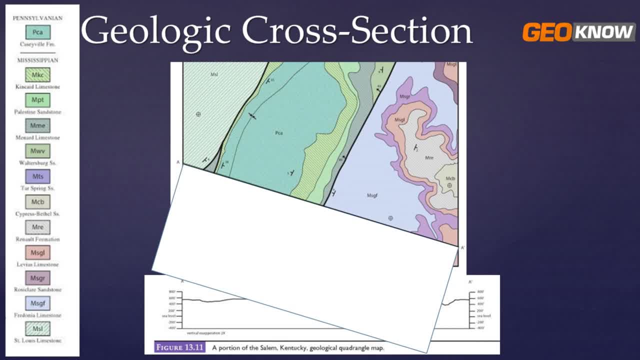 just either way, anytime you find a change in rocks which you'll see by the change in color. So if you look over here, we actually have a geologic column that's going to tell us a little bit about the rocks on this map. I will say a little disclaimer: here we don't have a lot of. 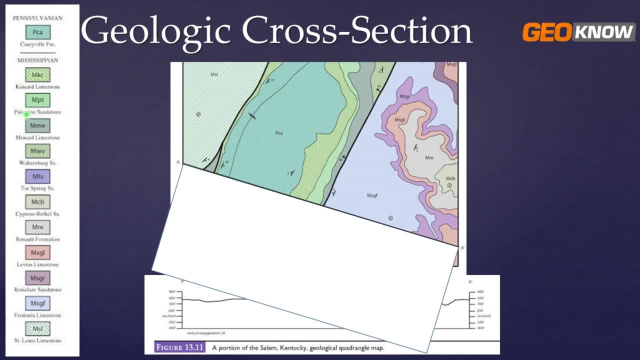 information just on these rocks. A lot of times you'll have a description underneath them that will give you information like thickness, and it'll tell you what the rock is going to look like. It'll give you a little bit about the rock unit. In this case, we don't have that, And so we're going to 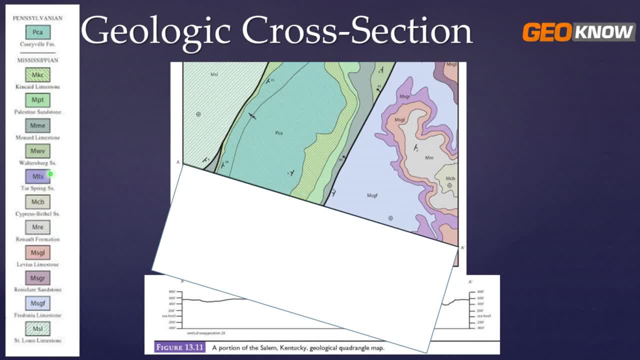 have to kind of do some guessing, do some guesswork and that kind of thing, But overall at least we have the pattern of the rock, matches what's on the map and we know the name of that rock. So, for example, MSL has this diagonal green stripe pattern and we can look down here and see that that is the. 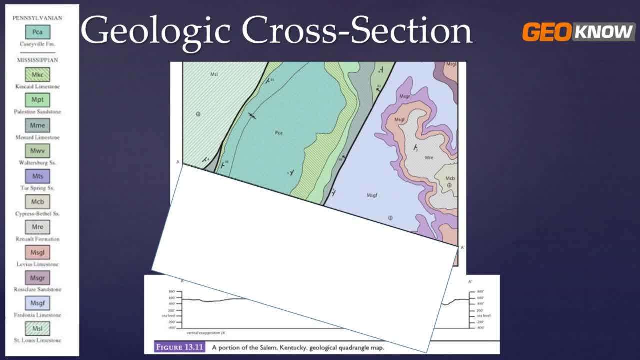 St Louis limestone. Back to drawing the geologic cross section. The first thing we hit it looks like those thick black lines are a fault. So we're going to draw just a little tick mark Just show us where something's happening. 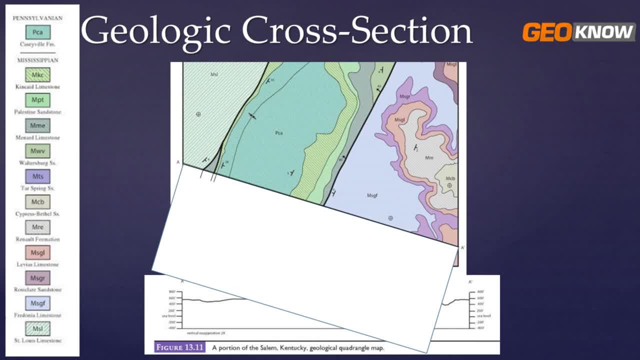 Next thing is another fault. And then we have a change in rock unit. So one thing I did not take into account in this video just for simplicity sake- but your teacher or instructor may require you to do so- is this line that runs down the page here, You notice. 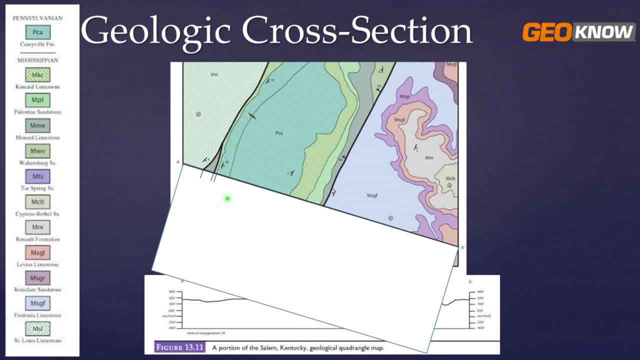 these two arrows. It's where the geologic feature here is converging. So you notice, here this little dip line is showing you which way, which direction the rocks are dipping. So here they're dipping to the right over. here they're dipping more to the left. 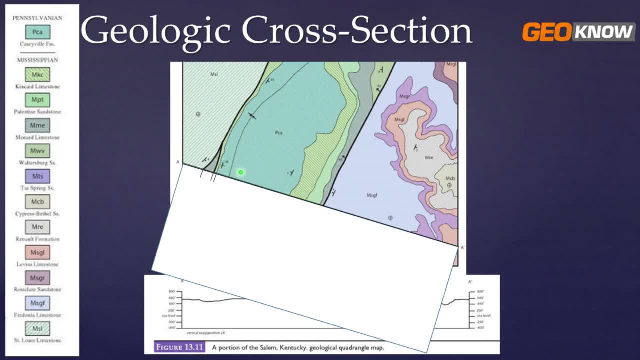 So if these ones are dipping this way and these ones are dipping this way, that means it's pretty much like a U shape, right? And what this line is indicating is where it switches from dipping one way to the other way. I did not. 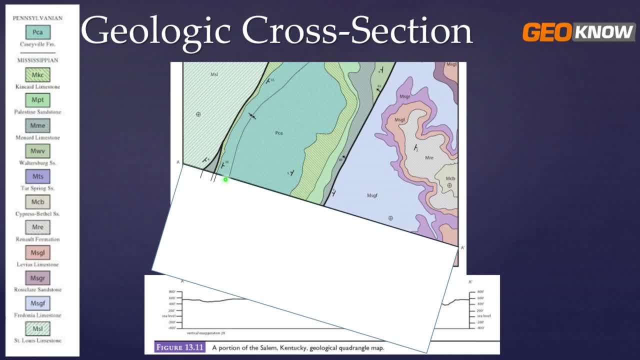 bother to take that into account. but just you know, if you have something like this on your map, make sure to ask your instructor If they want you to take that into account. Obviously, you're going to make a better map if you do that. 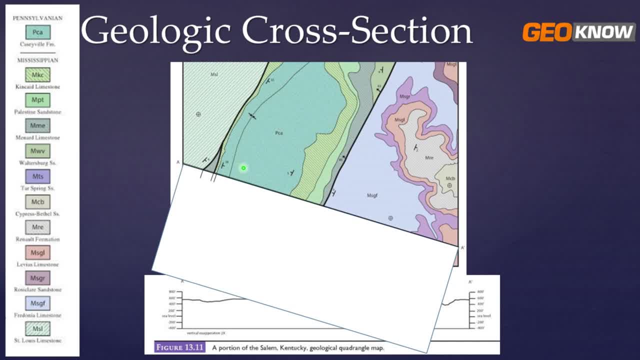 I was just. yeah, I neglected to take that into account before it was too late. So don't be like me. is the lesson of the story or the moral of the story? Anyway, we'll continue making our tick marks. So it wasn't a you know, we're. 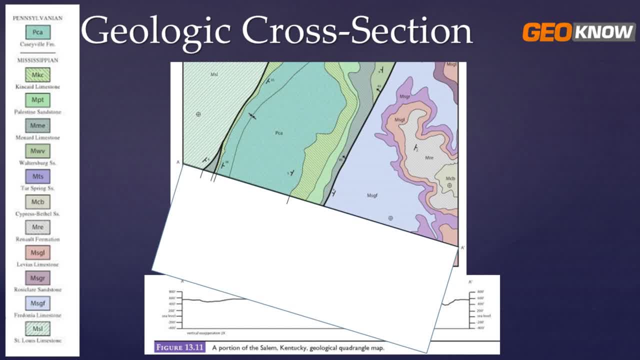 still the same rock unit from here to here, but then we changed to this kind of yellowish green diagonal line And then we change again. we change again another fault line, that thick black line, And notice the dip signature for faults is a little bit different. It's actually: 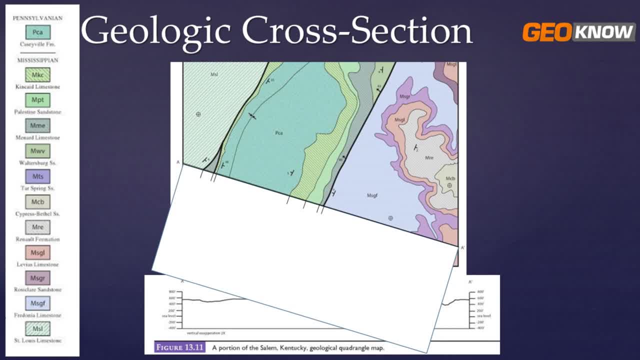 an arrow. It points in the direction that the fault is dipping and it tells you how many degrees it's dipping. And then we go, we continue on, we reach another change, another change and we find the end of our line. 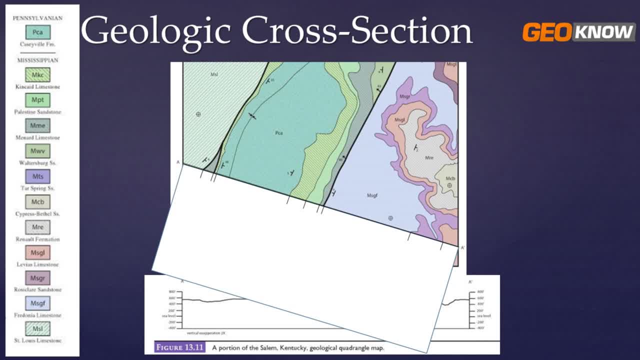 Now this little symbol with a plus and a circle. that actually means that the rocks there are more or less horizontal. They don't have any dip to them. Now we do see that. you know, there's a subtle dip here, like two degrees. 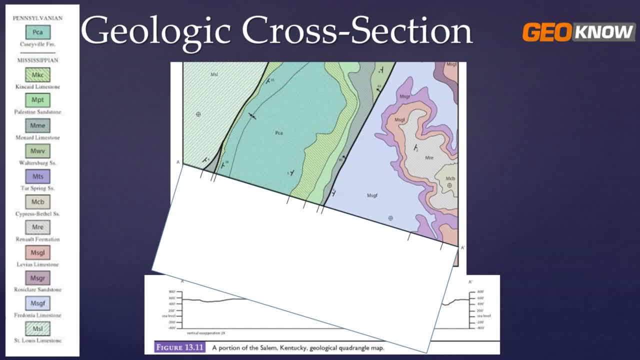 This is nine degrees. I'm guessing that was influenced by that fault. The fault kind of pulled the rocks down a little bit to make them a little steeper, But over here, you know, you just see that it gets pretty much just flat Maybe. 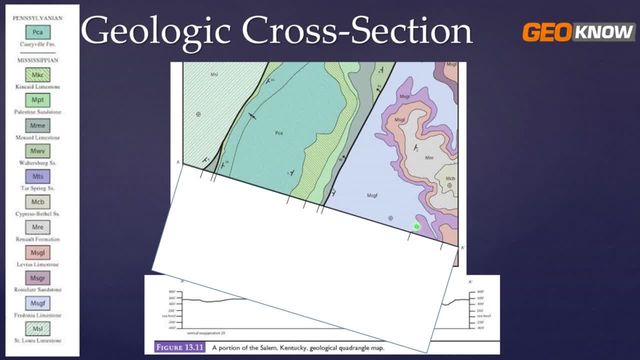 there's a two degree dip over here. We don't have a ton of information for this map, but we'll use what we can get. So once you've got those tick marks, you're going to take them to your little geologic topographic. 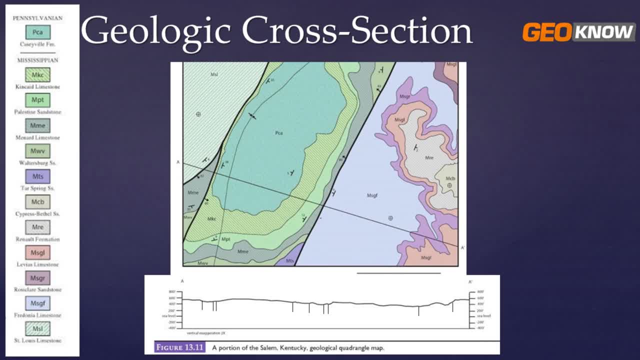 profile down below. In this case, they've actually given us the topographic profile. so what that means is from A to A prime. it's just showing the elevation of the surface. If you don't know how to construct a geologic cross-section, that's also going to be something. 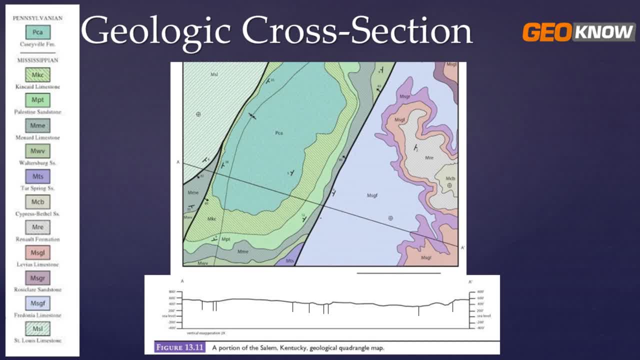 very important for you to know, And I'll leave a link in the description below so you can get a video that I created on how to create a topographic profile, because you may need to do both things in creating a cross-section, In this case. 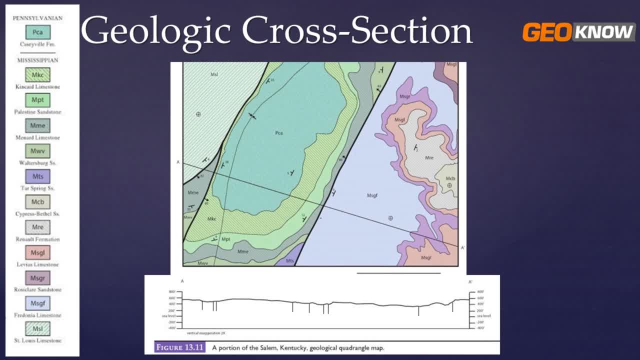 we're not going over that. They've already drawn it for us, so that was very nice. What I've done is I've transferred my tick marks, So I took my piece of paper and I lined them up with our little grid down here. 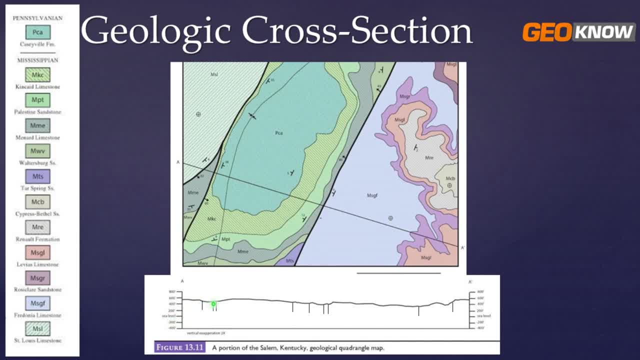 our little graph and I've just made a tick mark, just transferred my tick marks to the little grid down here. So this is that first fault, then the second fault, then that first little change in rock unit, another change in rock unit, etc. and so 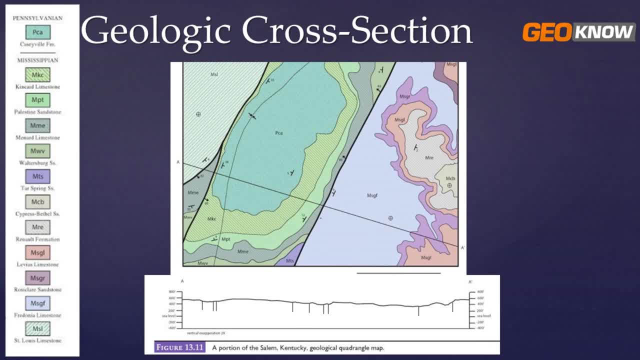 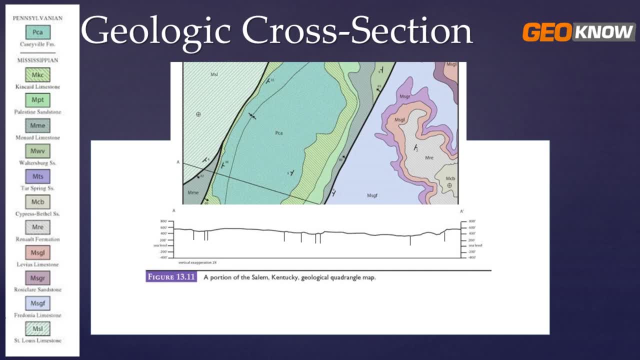 on and so forth, So we see where things are changing. So I'm just going to move up the topographic profile grid just because I don't have enough space and I need to be able to show you how to do this with the protractor. 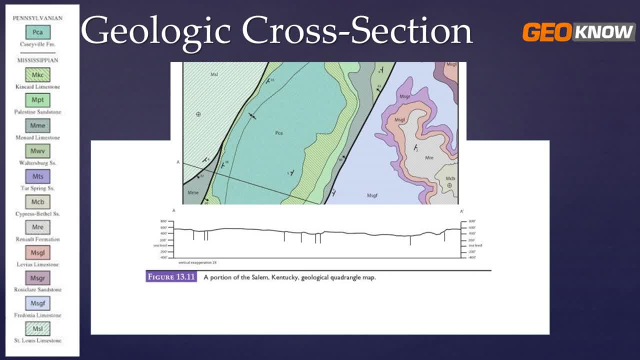 So you will need a protractor because you need to take into account the angle of things. So the first thing we have is the fault. And we look at the map and we look that it's dipping more or less kind of southeast, but for our purposes that's more or less. 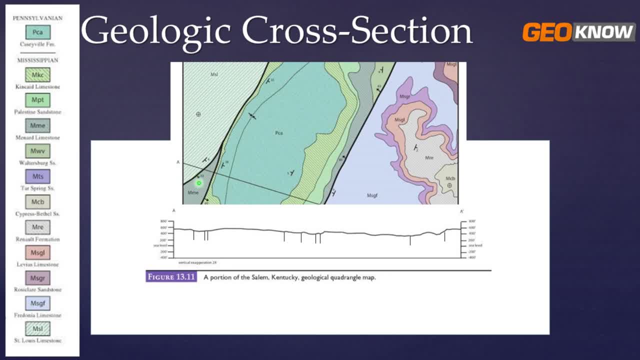 parallel with our line, So we'll call it 82 degrees dipping to the southeast or east. So we'll get our protractor line it up with that first mark. We need to get an angle, So 82 degrees to the southeast. 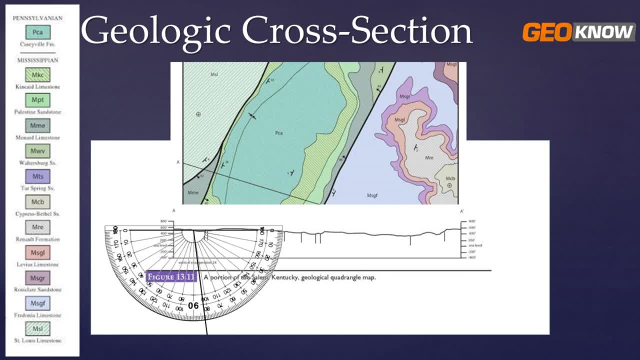 So we want to make sure we're pointing the right direction. 82 degrees, we've got it lined up. So in your case you're going to have probably a pencil. don't do this in pen, because you're going to need to erase some things. Make a little. 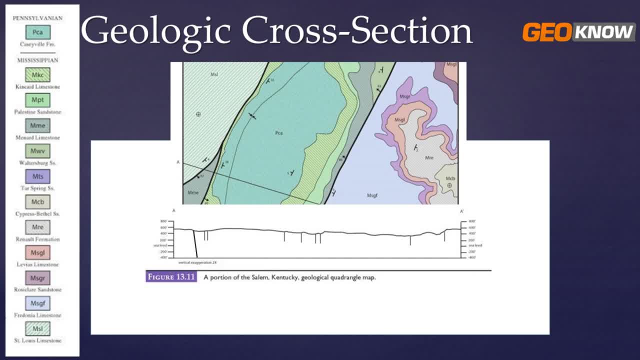 mark there at your 82 degrees and then leave and you can draw your line down. In this case, I'm just going to draw the fault all the way down. We don't have any information to know if that fault stops somewhere, But for simplicity's sake I'm just drawing. 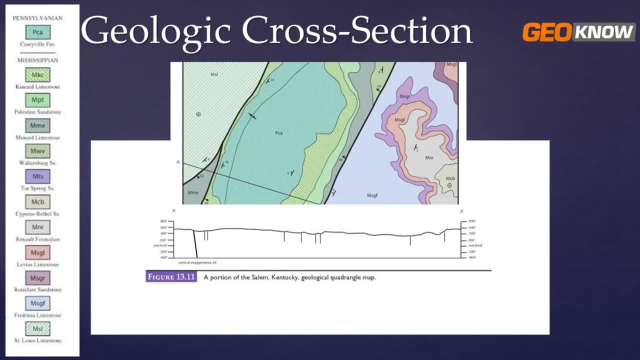 the fault all the way to the bottom of the page Or the bottom of the graph. So the next thing we come across is another fault, And in this case it's dipping the same direction, but it's dipping a little bit steeper. 85. 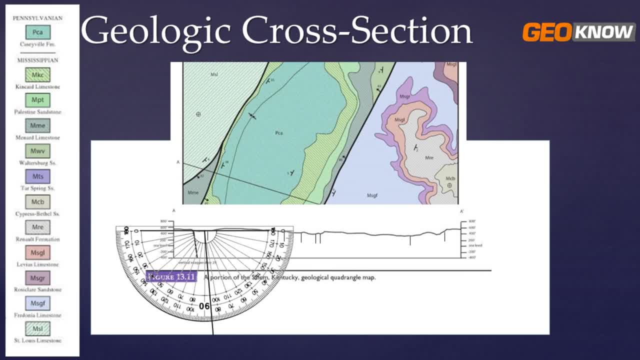 degrees instead of 82. So again, line up your protractor, Get an angle of 85 degrees And then draw your little line of 85 degrees on there. It's going to be a little different for you. I get that because 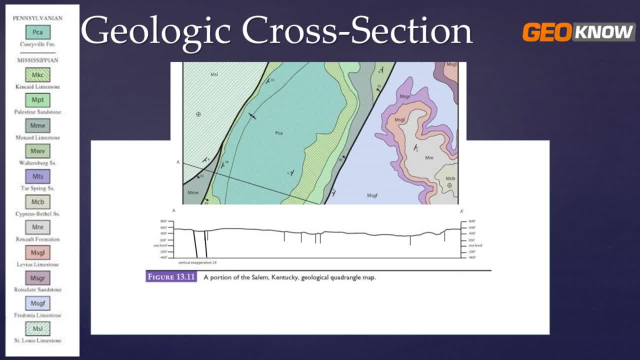 you're using paper, I'm using powerpoint, But hopefully you'll be able to figure that out And feel free at any time. pause the video, ask a question down below. I'll do my best to get back to you and answer those questions. 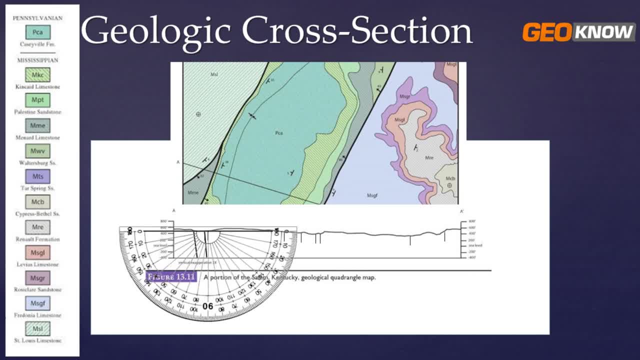 Alright, the next line. So we come across this unit here, This green polka dot unit. So we look over here, That's the youngest one on our map. We can tell it's the youngest because it's the one that's on top And that's how geologic. 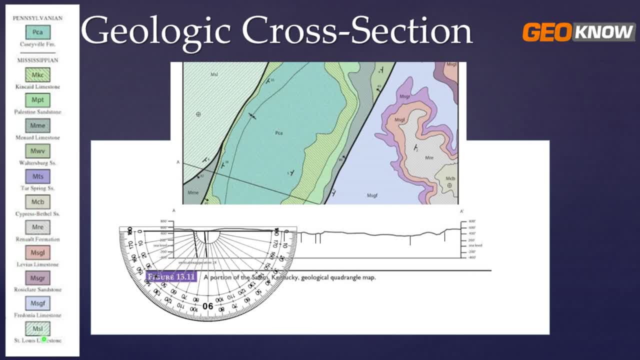 columns usually are from top to bottom, Youngest to oldest. So we've got our youngest unit And it is dipping to the east more or less parallel with our line, And it is about 35 degrees to the east. So we're going to draw. 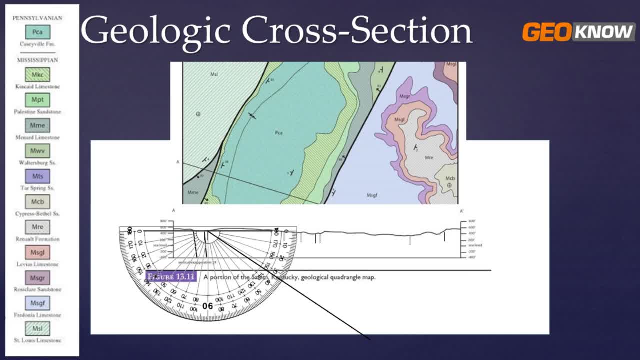 a line About 35 degrees dipping. And there we go, There's our line. So we know those rocks are dipping that way, at that angle. Alright, let's go to the next line, Get our protractor all set up. And we know that these rocks- 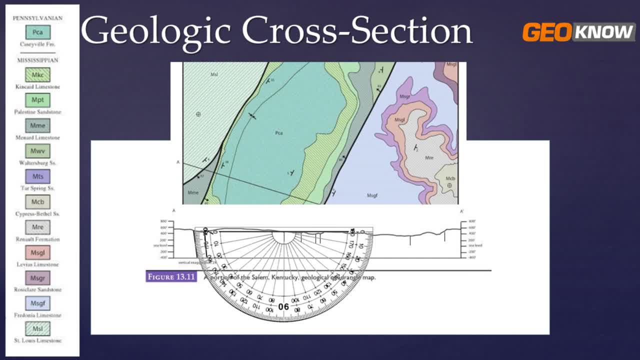 are dipping the other way right. So these are dipping more west ward, And this is only a 5 degree dip, so it's much more shallow. But anyway, we still measure our degrees. And here we go. There's our degree dip. 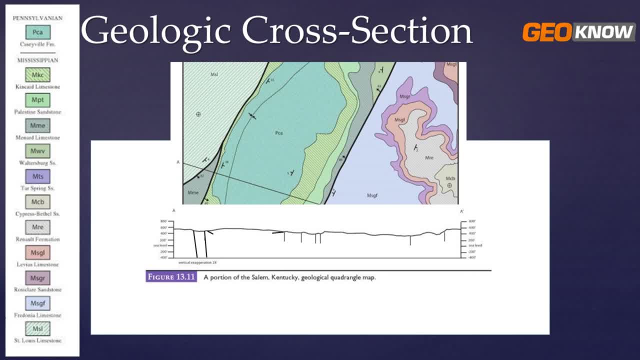 Now I do want to emphasize once again when you're drawing these lines together. So we know that these are the same rock units, so these two lines should match up at some point. What I again, what I failed to take into account, was this: 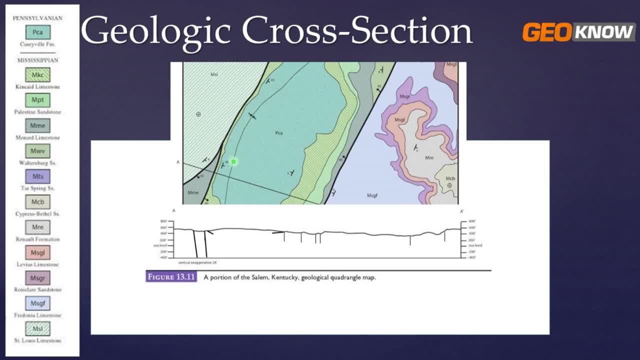 inflection point where it changes from dipping one way to the other, which we should have taken into account more or less right here. But again, I won't bother saying this again, but I did not take into account to do that on this map. 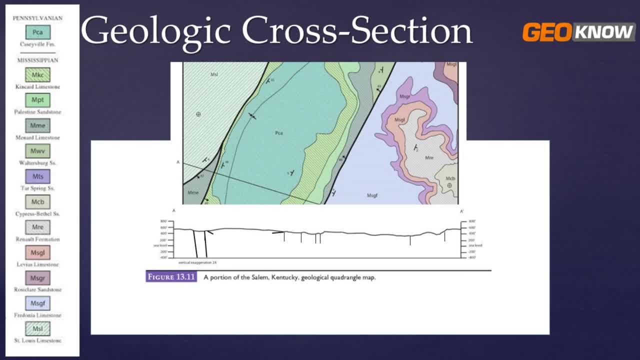 So just keep in mind that my drawing from one point to the other is not perfectly accurate, given all the information that we have. But there you go, We go ahead, we draw the two lines together. Yours will look better than mine because you'll actually do it right. 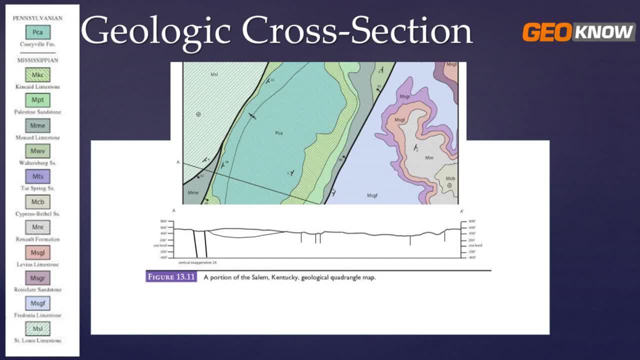 Alright, moving on to the next unit. So we know this one. we don't have a lot of information for this one actually, So we don't. I don't think we have a dip angle for it, But we do know that there's kind of a 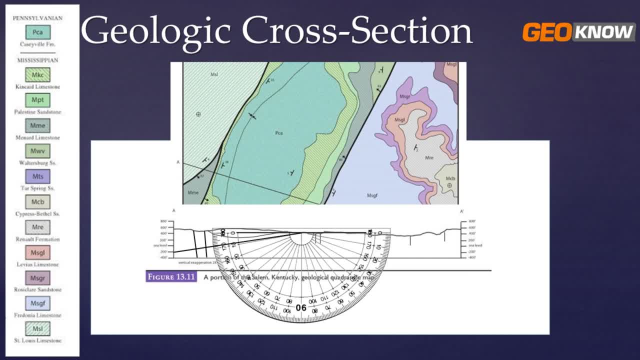 12-ish to 5-ish angle. so I'm just going to pick 9 degrees, just somewhere in that range, since we don't have an official number And we've got our line lined up, There's our little tick mark. And since 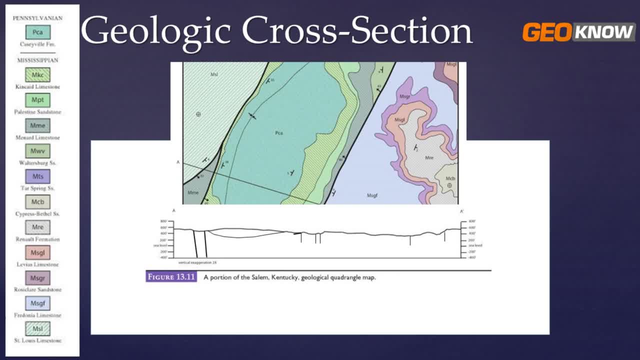 there's no reason to suggest otherwise. the best guess is that the rocks below follow the pattern of the rocks above, So we can just kind of draw a line in following a similar pattern to the rocks above. Now, if there was a fault or if we were, 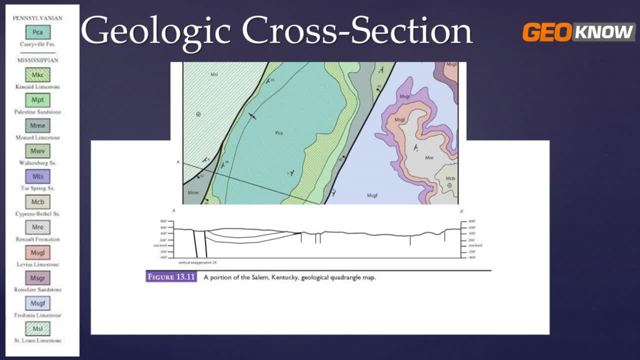 told there was an unconformity of some kind, which that's another discussion for another day. we'd have to take that into account. Alright, so let's take a look at our map again, This green unit: here we do actually have a dip. 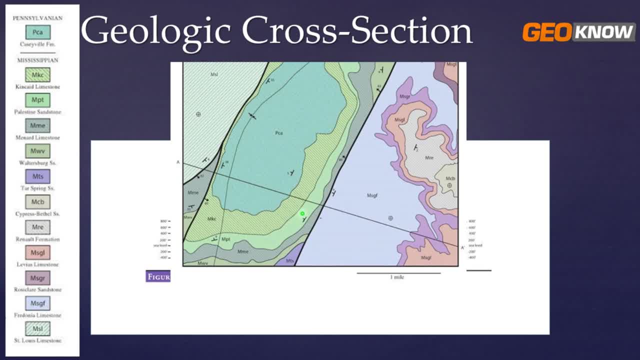 symbol on this and it's heading westward about 12 degree dip. So we'll use that information and draw our next point: Get your protractor out, draw 12 degree. You make your little tick mark there and draw in your line. 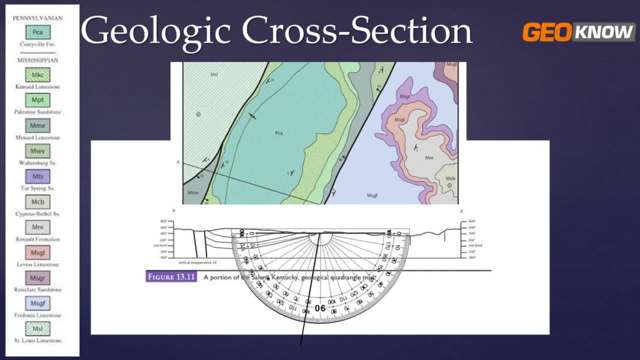 We don't have any information on that gray striped rock unit which is the Menard limestone over here. We don't have any dip information on that, So we're just going to have to come back to that and more or less draw it in as a similar. 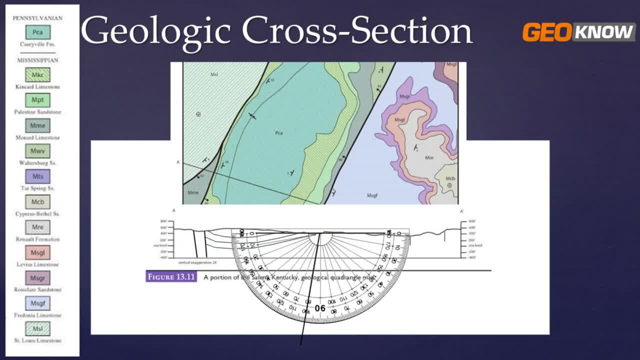 pattern to these other rocks. But for now we're going to focus on our fault. So our fault, we know, is dipping kind of northwest but west, you know, more or less parallel with our A to A prime line, and it's dipping at 80. 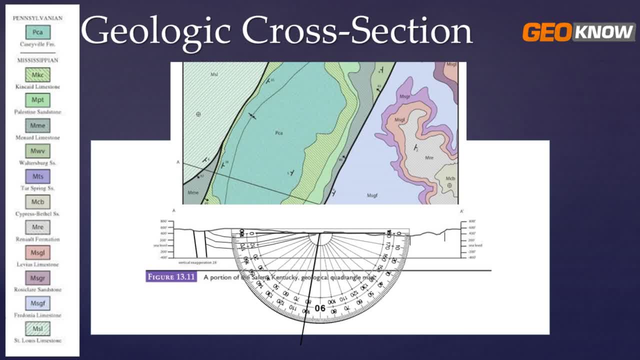 degrees. So I've got my line angle 80 degrees, but the other direction than those other faults were. And there we go, Gone ahead and drawn my fault in. So what I'll do now is just draw the rest of the rock units. 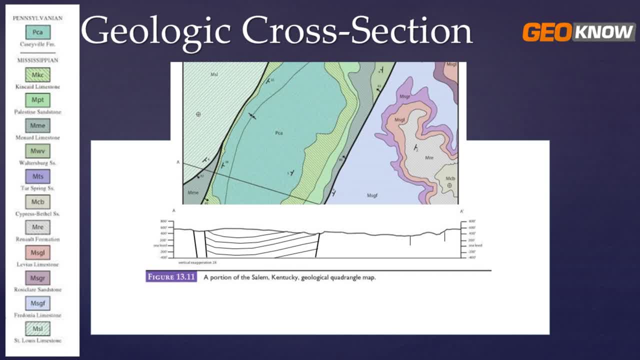 in. The problem here that you want to keep in mind is I had to do a bit of guesswork because, again, we don't have any information on the thickness of these units. So, for example, if we were told that the Menard 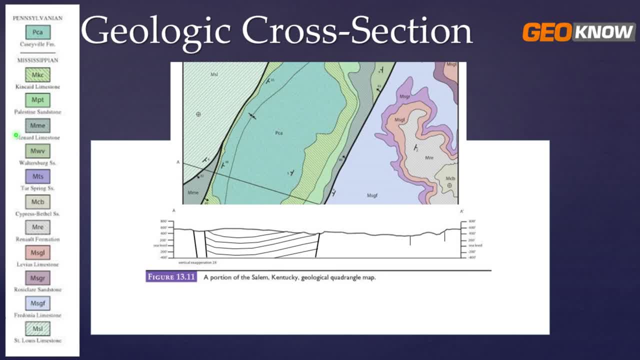 limestone was like 200 feet thick or 500 feet thick. that would help us determine how thick to draw these units here. You could use this scale on the side to measure the right thickness In this case. I'm just guessing because I don't. 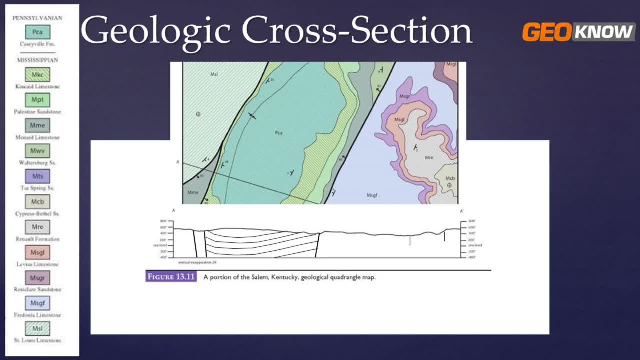 have that information. Most likely you will, and if you don't ask your instructor what they would like you to do in that case, Alright. So here we go again. If we're traveling this line, so we just did this fault, the next thing we can. 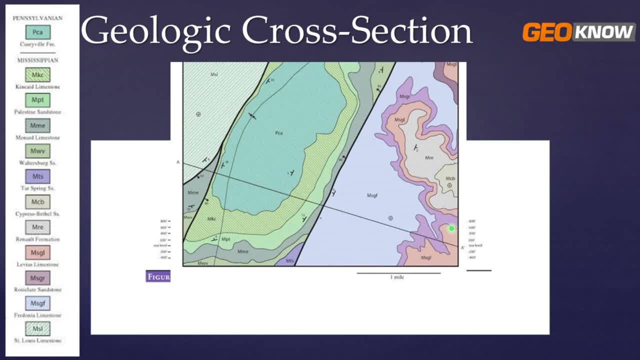 encounter are these light purple, purple and kind of salmon colored rock units. So if we look over at our geologic column, we're at the Fredonia limestone, the Rosiclair sandstone and the Levias limestone. So we know that the 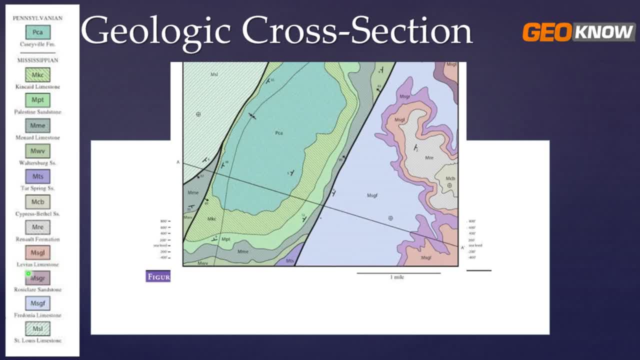 Rosiclair and Levias are younger units so they should be on top of that purple unit, And we also know that the dip is not very significant here, but we may put it at like a two degree dip just because some of these rock units are shown. 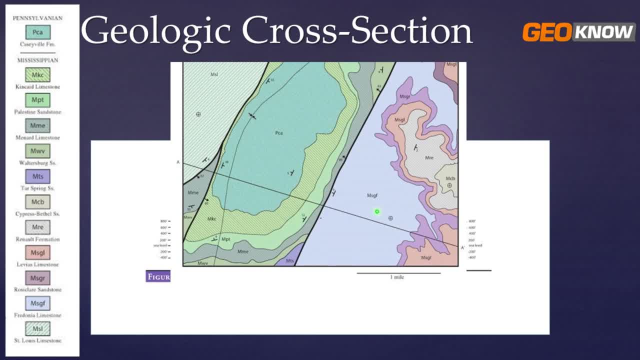 that Over here, though, it should be more or less flat. So those are just some things to keep in mind. Over here, there's a little bit of a dip, I think. again, it's just close to that fault, so the fault's dragging. 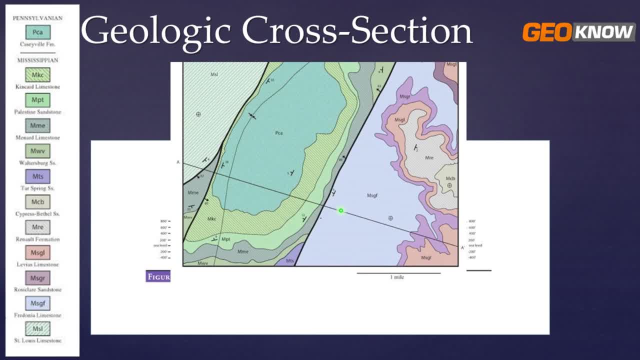 the rocks down a little bit and causing them to dip. But over here it's flat, And so we're going to make marks where those other units are. I did draw them with a little bit of a dip and I projected this line out just so you could see. So if we did project 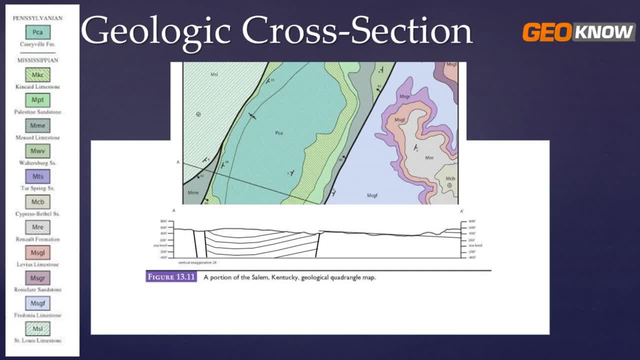 that rock unit out. we could explain why we're not showing it over here, where the surface is a little bit higher. Why are we not showing it on the map? Well, that's because it's all been eroded away. So all we're seeing is that. 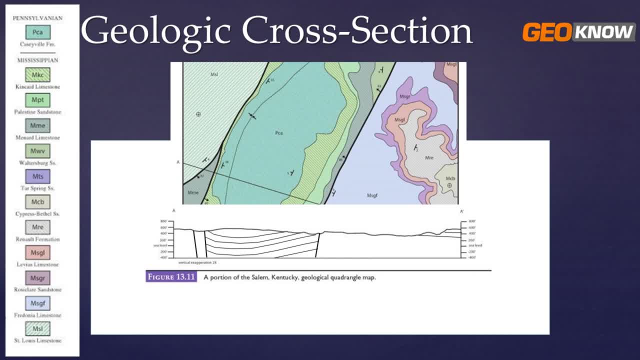 Fredonia limestone. Alright, so we've got that under control. Now we just need to. I need like a nine degree dip, just for reference. So I'm just this is just how I'm doing it. I'm just drawing a nine degree dip. 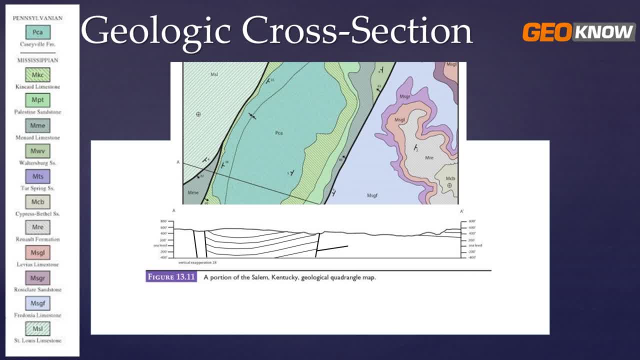 line and I'm going to place it somewhere on this side of things and I'm going to use it just as a reference so I can draw a nine degree dip. You could actually just use your protractor And again, we don't know the thickness of this unit. 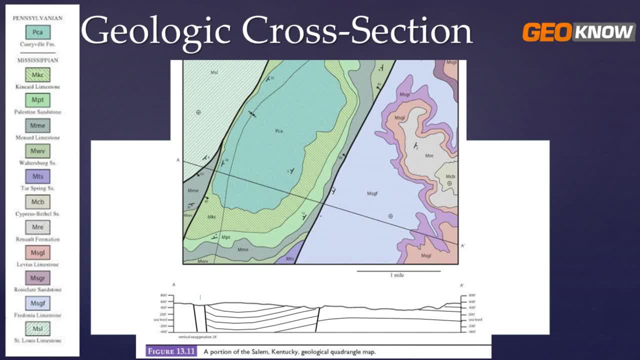 So I'm just going to have to draw it in. So notice, I've got that nine degree dip over here by the fault, And it comes up more or less flat where we have that little plus symbol inside a circle, And then I just had it have a slight dip. 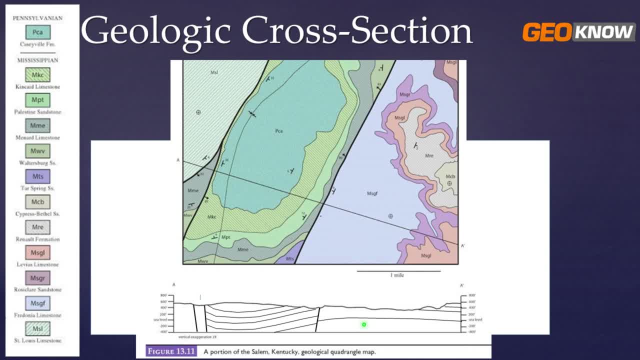 just like the other rock units, Just to follow those. Now we don't really have much else to draw under this other than the St Louis limestone, but under that we don't really know what's under there, So we need to draw that. 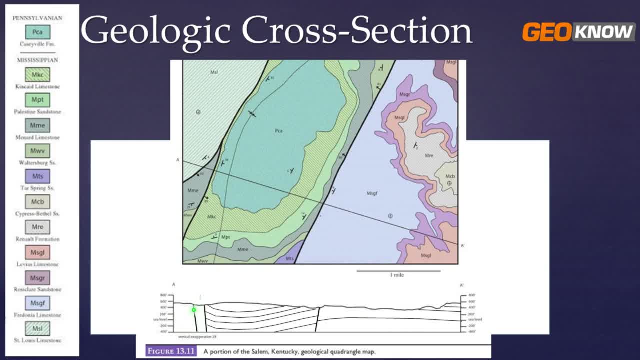 St Louis limestone in and we need to go back and fill in these areas that we've left. So in those areas over there, we know that these, this limestone here, this Menard limestone, is dipping at about 35 degrees. 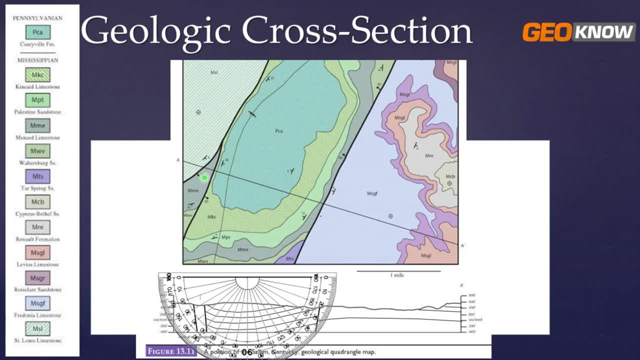 So that's just the degrees I'm going to use. That may not be perfectly accurate because it is dipping in a slightly different direction than our line's going, but we'll use that just because that's the information we have. So 35 degrees. 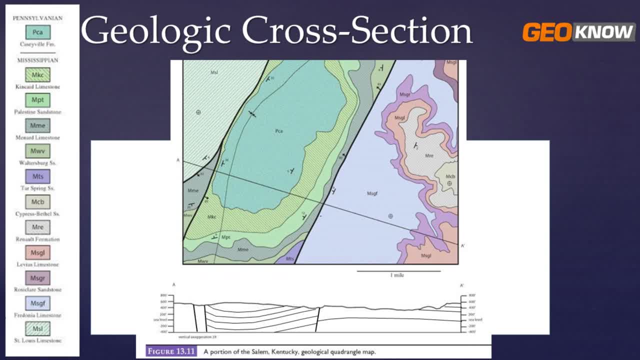 I'm just using that again as my angle. You're going to have to do this a little bit differently on paper for obvious reasons, But then we're just going to draw in the units below it. So we have our Menard limestone, then our 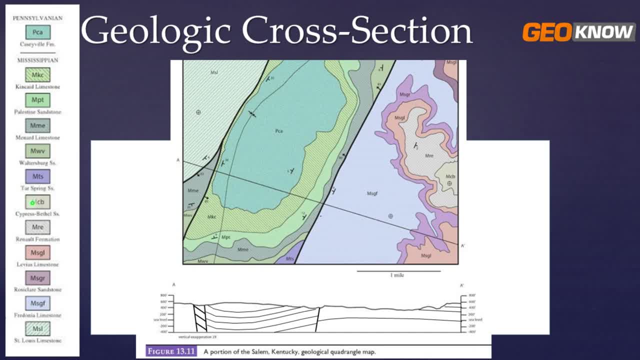 Waltersburg sandstone, Tar Spring sandstone, Cypress Bethel sandstone, etc. etc. So those are the units that you'll expect to be underneath the Menard limestone. Now, this last little section is a little trickier. It's more or less flat, a little bit of. 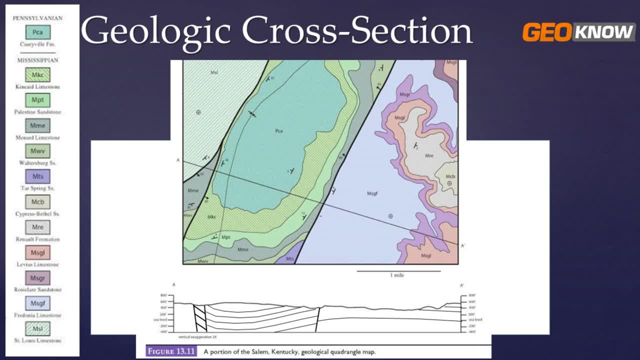 a dip by this fault. You know, again, I think the fault's kind of dragging it down. Get our protractor out, just so. we have a 4 degree dip, to be sure. And since we're pretty close to that fault all the way on our little cross section, 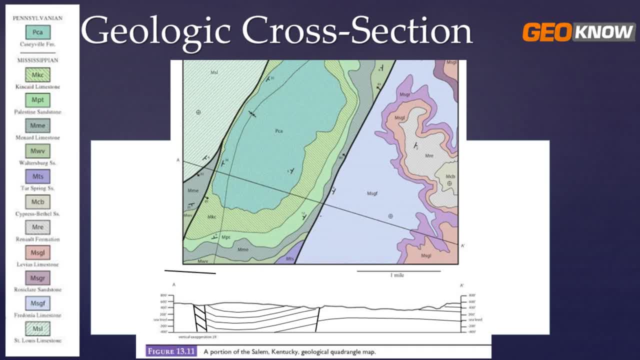 I'm just going to keep the whole thing 4 degrees. So there's a 4 degree line right there. I just used the protractor to draw that. Now here is the tricky part. We don't know anything about any of the rock units or what's going on below the 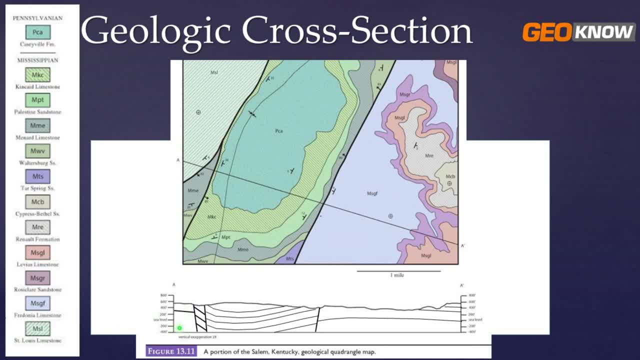 St Louis limestone. So I'm pretty much just going to draw a question mark underneath that. That normally would not be appropriate because you would have more information like thickness of the unit or something like that, And could I go look that up? Yes, But I'm trying to show you. 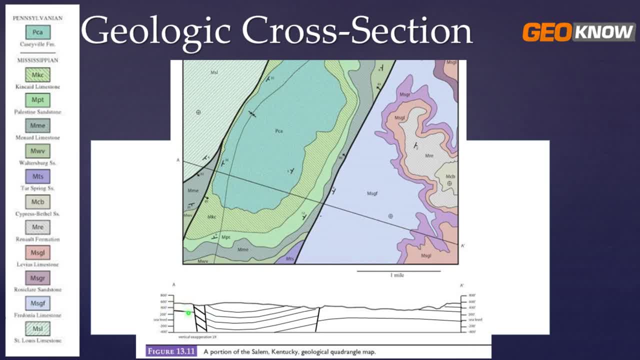 how to draw a geologic cross section, and that's about all I'm trying to do here. So there you go. You more or less have a cross section there. What's left is just to draw or color it in, And that is what it looks like, more or less. 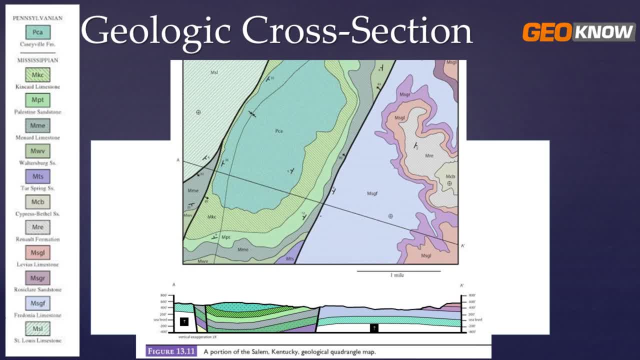 colored in. I had to more or less kind of improvise a little bit with some of these units, just using what PowerPoint had available for patterns and colors. I tried to match them to what was up here, but maybe it's not perfect. But there you go, That is. 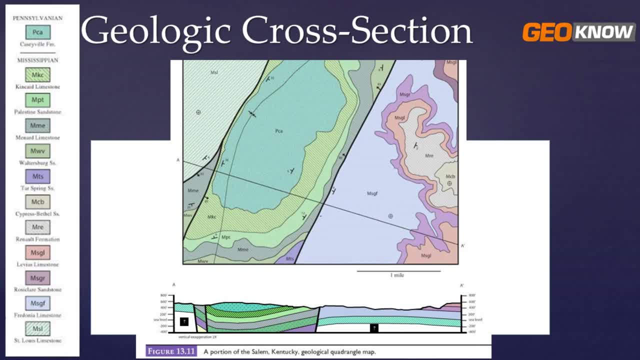 a geologic cross section based on the information that we have on that surface of the map. So hopefully that's helpful to you guys. Let me know what you guys think. Did I make any mistakes? What would you do differently? You could tell me that too. 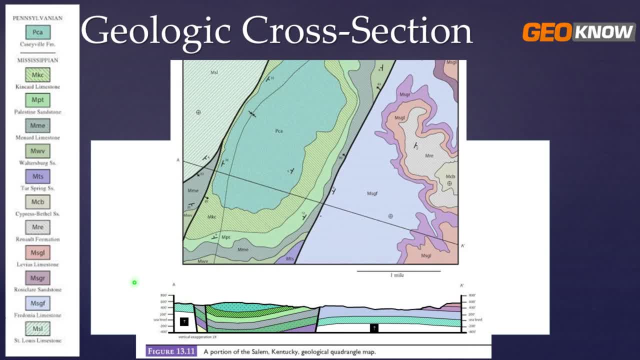 If you have any questions, let me know. But again, it's always good to get the expectation of your instructor as to what they want you to do in these strange circumstances where you don't have enough information. You know, I could have just assumed that the